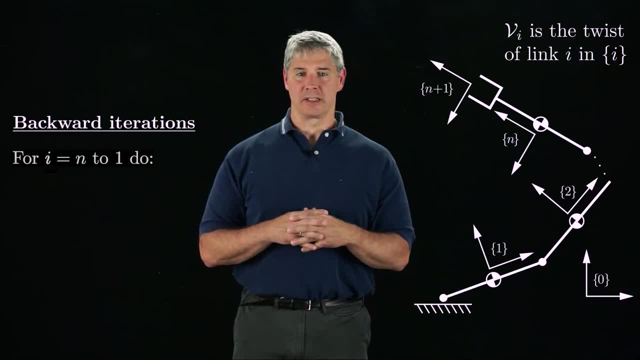 of each link. Now we perform the backward iterations, calculating the required joint forces and torques, starting from joint N and moving backward to joint 1.. First we calculate the wrench fi required for link i as the sum of the wrench fi plus. 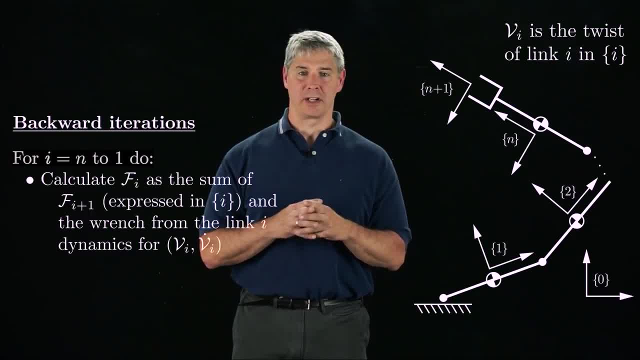 1,, which is the wrench needed at link i, plus 1,, but expressed in the i-frame, plus the wrench needed to accelerate link i using the inverse dynamics of a rigid body derived in the previous video. Then we calculate tau i as the component of the wrench fi along the joint screw axis. 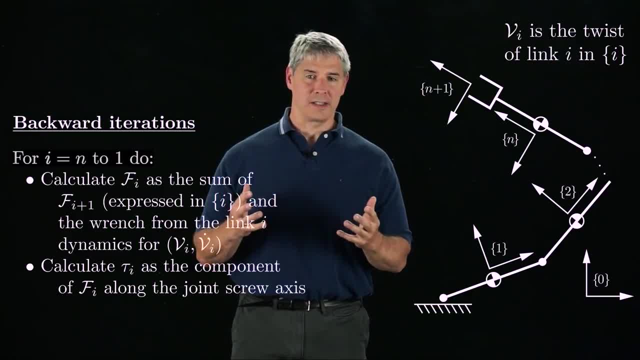 Only that portion of the wrench has to be applied by the joint motor. The rest of the wrench is provided passively by the mechanical structure of the joint, such as the bearings. At the end of the backward iterations we have calculated all the joint forces and torques needed to create the desired joint accelerations. 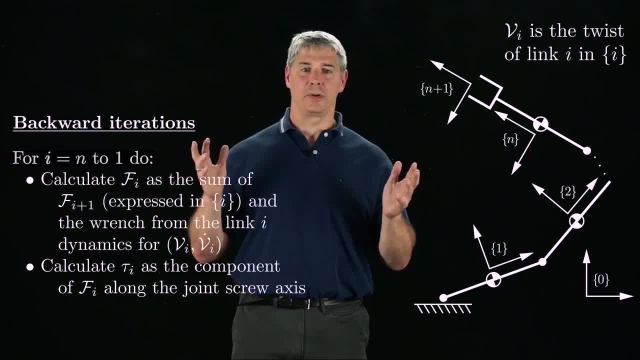 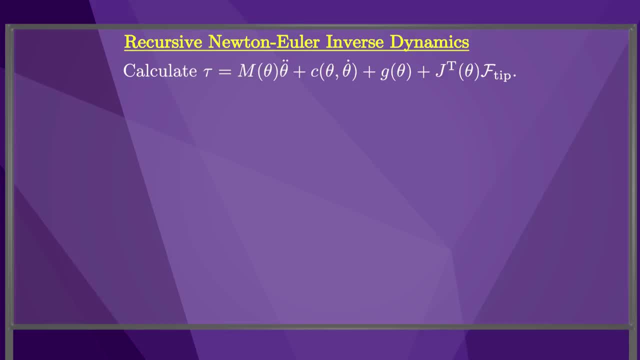 at the current joint positions and velocities. That's all there is to it. The rest of this video is just filling in the details. So, formally, the recursive Newton-Euler inverse dynamics algorithm calculates tau given the joint positions, velocities and accelerations, as well as the wrench f-tip that the robot 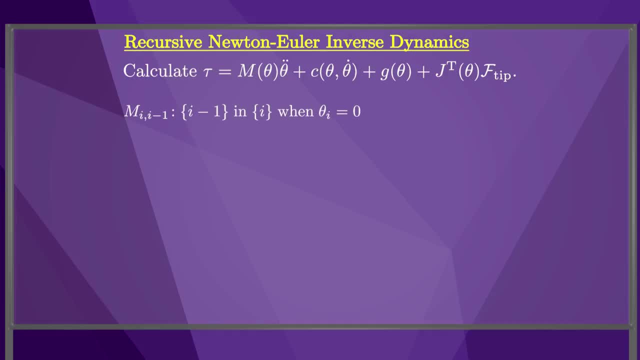 end effector applies to the environment. We define mi i minus 1 to be the transform defining the frame i minus 1 relative to frame i when joint i is at its zero position. We define ai to be the screw axis of joint i expressed in the frame i. 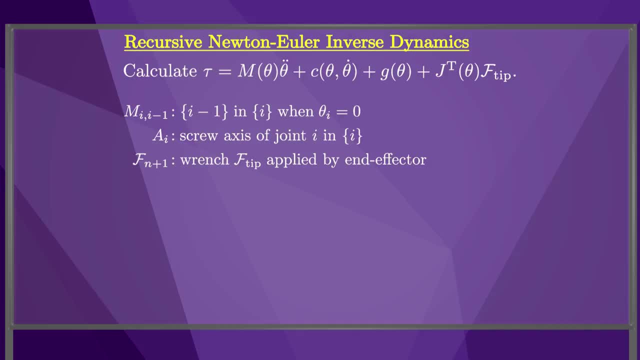 We define the wrench fn plus 1 to be the wrench f-tip applied by the end effector. Finally, to model gravity, we define the acceleration of the base of the robot v0 dot to be a linear acceleration opposite the gravity vector. 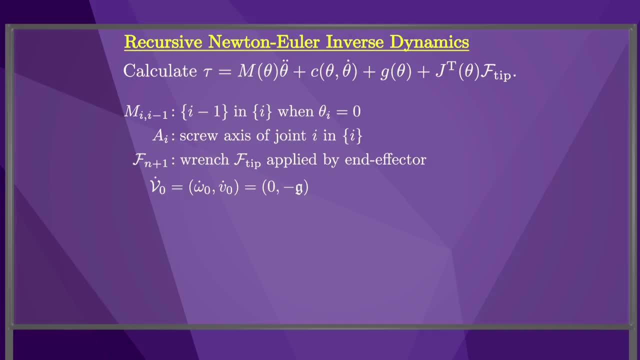 This is because gravity is indistinguishable from upward acceleration. In other definitions, the forward iterations from frame 1 to frame n can be written as follows. First, the configuration of frame i minus 1 relative to frame i is given by the formula: 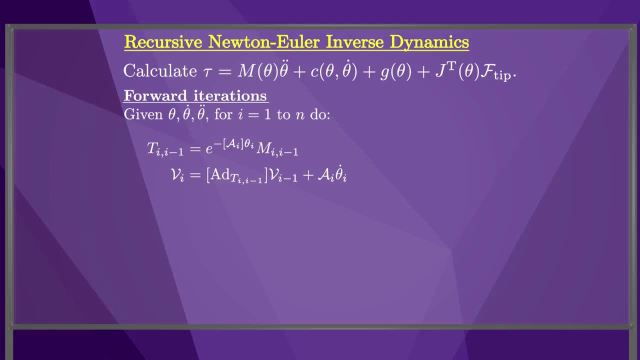 shown here. Next, the twist of link i is the sum of the twist of link i minus 1, but expressed in the frame i using the matrix adjoint of ti i minus 1, calculated in the first step, plus the added twist due to the joint velocity. theta i dot times the joint screw axis ai. 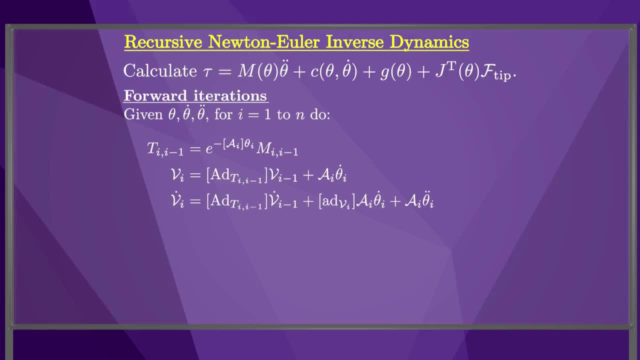 Finally, the acceleration of link i is the sum of the acceleration of link i minus x, expressed in the i frame, plus an acceleration due to a velocity product term consisting of the Lie bracket of the twist VI from the previous step and the joint velocity times. 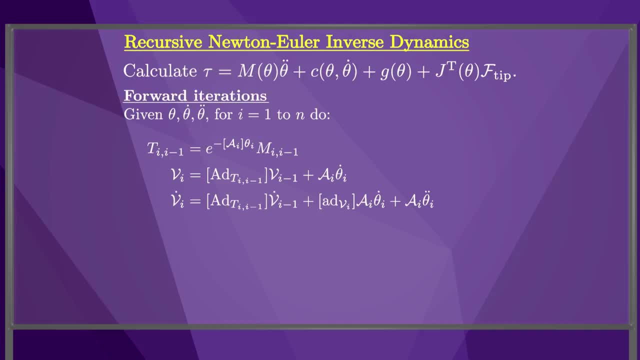 the joint screw axis ai, plus an added acceleration of the joint acceleration times the joint screw axis ai. The derivations of these equations can be found in the book. At the end of the forward iterations we have the configuration for the Ross-Sebastian equation. 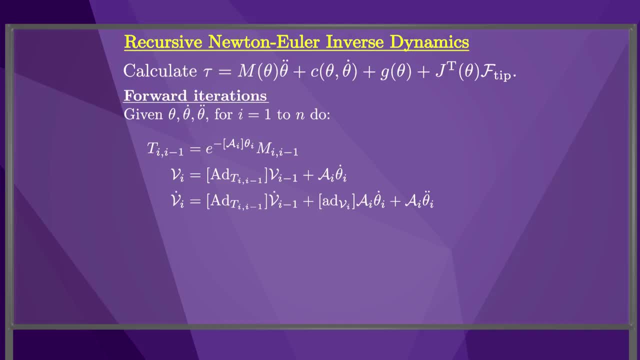 Debuchstein from Einstein's ratio and repairs succeeded. Sum completed, The result is snowaissee. Here's what about incredible denenvdas, moderating limitations and which the yearsも twists and accelerations. of all the links, The twists and accelerations are expressed. 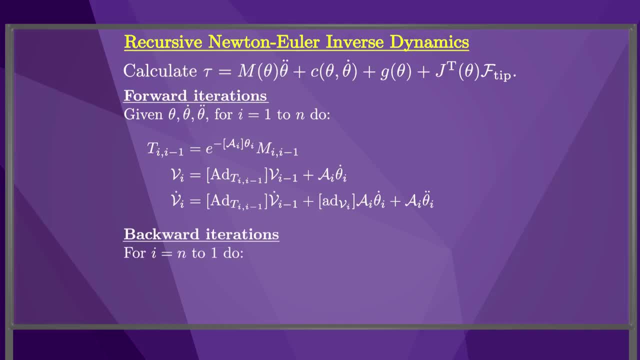 in the center of mass frames I. Now we begin the backward iterations from frame N to frame one. First we calculate the wrench Fi required by link I as the sum of the wrench required by link I plus one, but expressed in frame I. 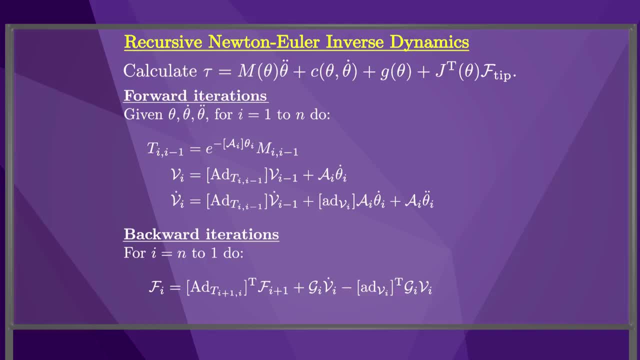 plus the wrench required by link I, according to the inverse dynamics of a rigid body we derived in the previous video. Finally, we calculate the joint torque tau I by projecting the wrench Fi onto the screw axis Ai. We now have the vector tau of all joint forces and torques. 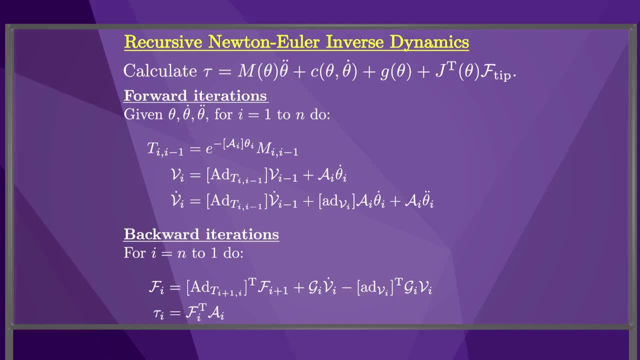 needed for a given theta, theta, dot, theta, double dot and end-effector wrench F tip. One advantage of this algorithm is that it involves no differentiation. Another is that it is computationally efficient due to its recursive nature, where calculation of link I's twist and acceleration. 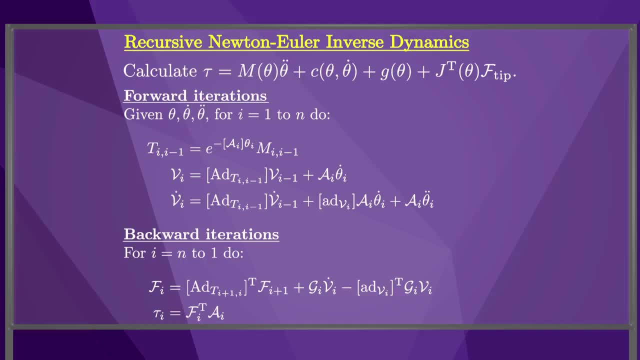 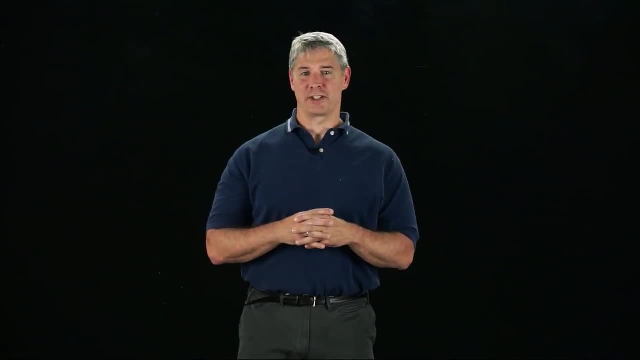 uses link I minus one plus one's twist and acceleration and calculation of link I's wrench and joint torque uses link I plus one's wrench and joint torque. The inverse dynamics are useful for robot control For simulation. however, we need to solve the forward dynamics. 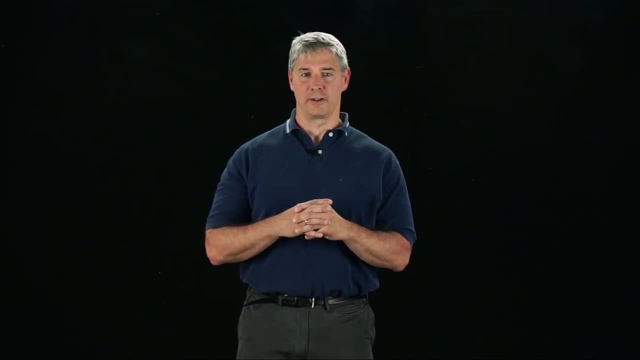 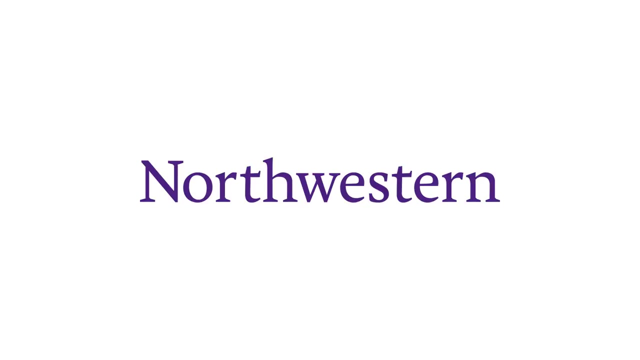 In the next video I'll demonstrate one way to use the Newton-Euler inverse dynamics algorithm to solve the forward dynamics. Thank you.